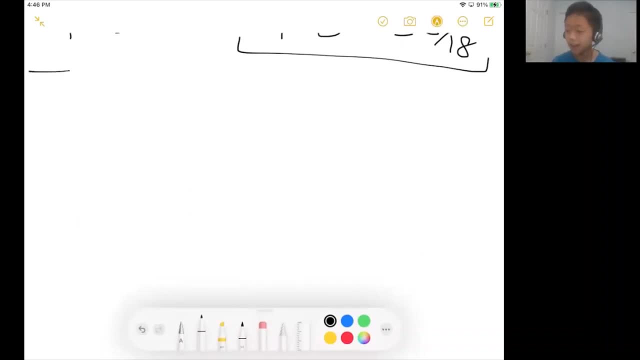 Basically says: we have four green marbles, four green marbles and three red marbles in a bag and we are going to select two marbles from this bag without replacement. So select two marbles from the bag without replacement and we want to find the probability. 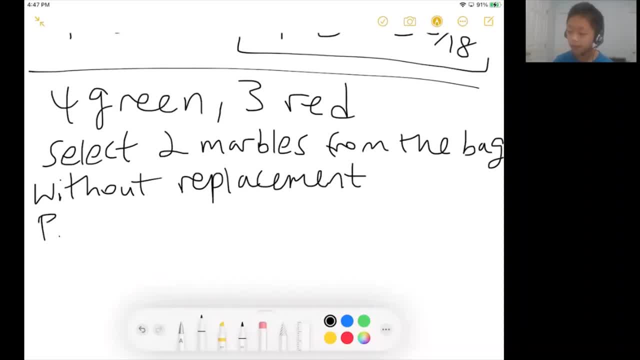 So we want to know what is the probability that we get two red marbles. So basically, first for this problem, maybe one of the important things to notice is the word like without replacement. So you'll see this a lot in math competitions. Without replacement just basically means you're not going to replace the thing that you like. 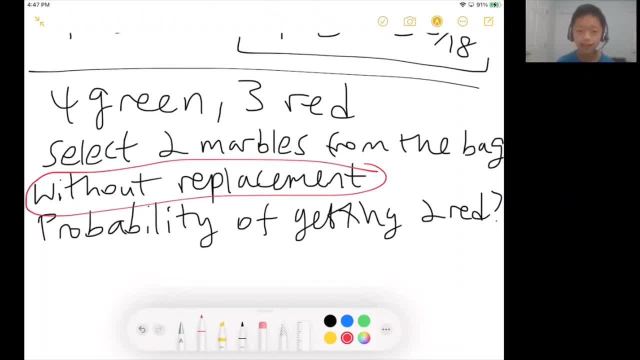 So if I draw a green marble, let's say I first draw a marble, I'm not going to put the marble back into the bag, I'm going to keep the marble and I'm going to continue drawing. If, on the other hand, if the question says with replacement, it means, let's say, I chose a green marble. 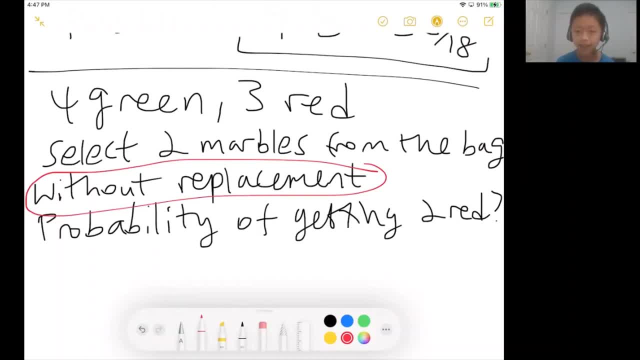 I'm going to take a look at the marble and I see it's green and I'm going to put it back into the bag, So I'm going to replace it back into the bag. So it's important to like be careful if the problem says without replacement, which means you don't replace the object that you took. 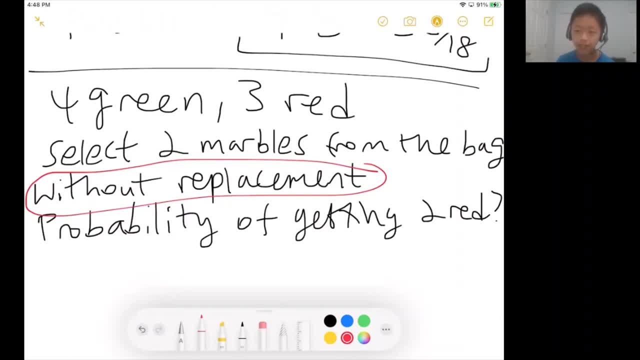 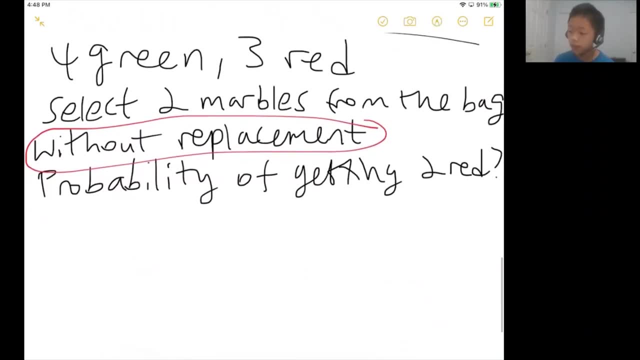 Or with replacement, which means you do replace the object that you took, And we want to know the probability of getting two red marbles. So this problem is pretty similar to the previous problem. So what we would do is, again like probability would be the number of successes divided by the number of possible outcomes. 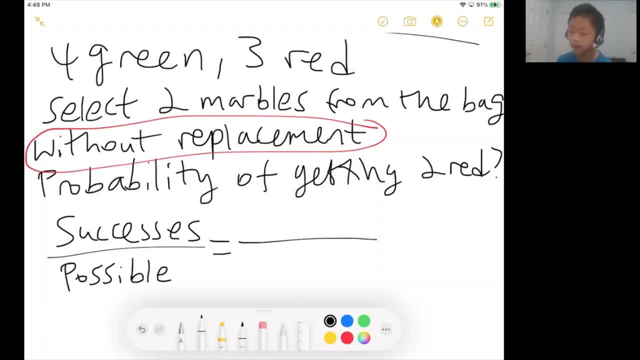 So the number of possible outcomes is going to be. there are seven marbles total in the bag Because four green, three red. So if we were to say that order didn't matter, then we would just do seven, choose two. And for the successes, since we have three red marbles, we want to choose two of the red marbles.